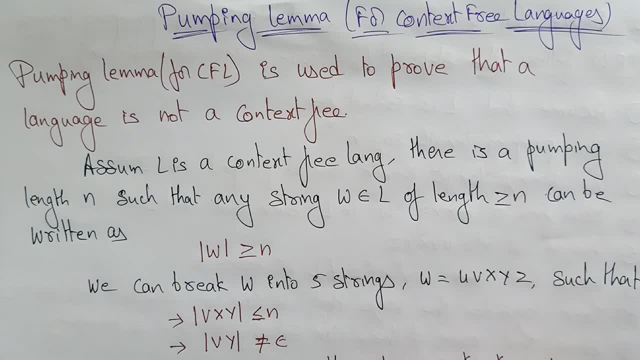 language or the context-free language that you need to be checked. okay, So in the previous video I explained means. in the previous videos, the starting of this subject, I explained about the pumping lemma for the context, not for the regular languages, regular grammar. Now, 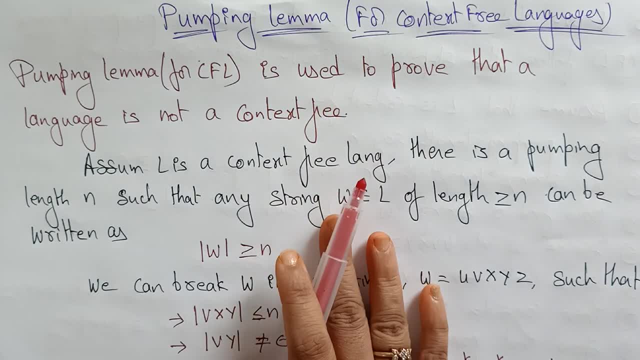 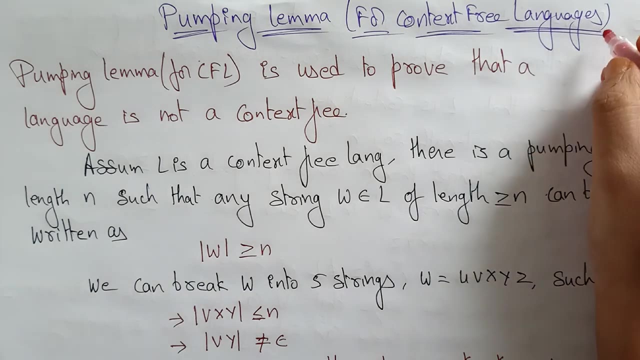 in this video I won't explain you about the pumping lemma for context-free language. So before going to know about the pumping lemma for the context-free languages, just recall what is a context-free language. okay, A context-free language is a language which is generated. the context-free grammar 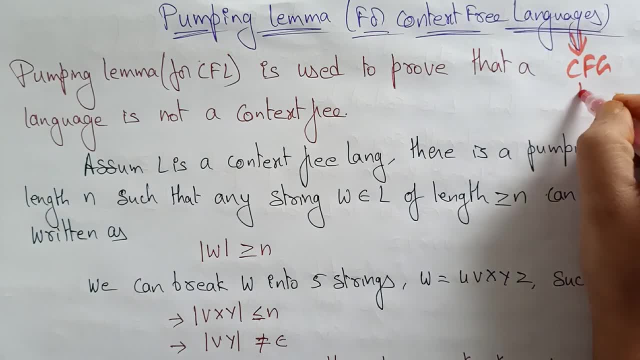 So this context-free language is generating context-free grammar. You already know that the context-free grammar consisting of four tuples. okay, It's consisting of four tuples. The four tuples are nothing but V, Sigma, S, P. These are the four tuples, which is 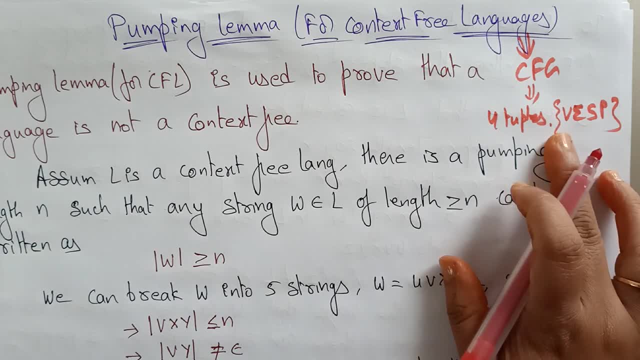 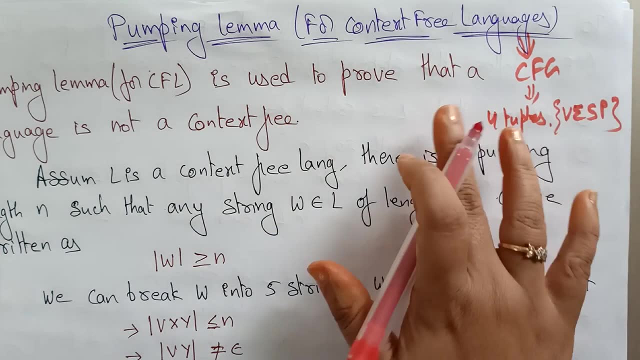 the context-free grammar consisting of V is nothing but the non-terminal set of non-terminal. Sigma is the input symbols and S is the start symbol and P is the production rules. That is the definition of the context-free grammar. okay, A context-free language is a language which 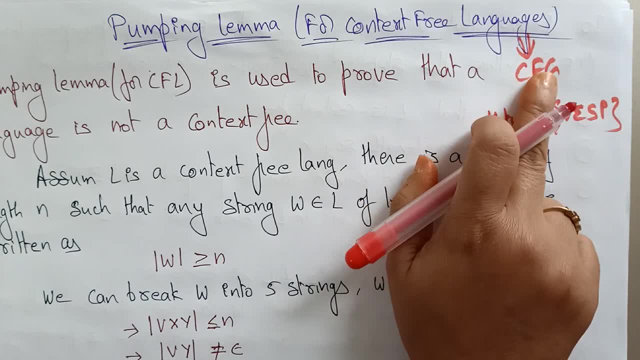 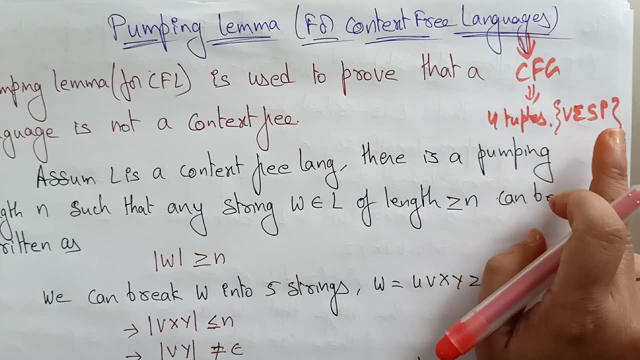 is generated some of the context-free grammars. The context-free grammars is defined as a four tuples: V, Sigma, S, P. V is a set of non-terminal. Sigma is the input symbols, S is a start symbol and P is a production. 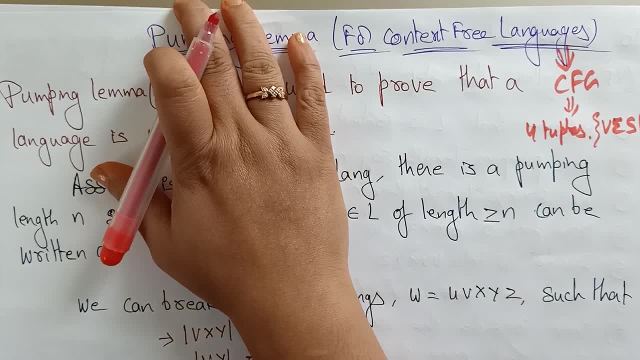 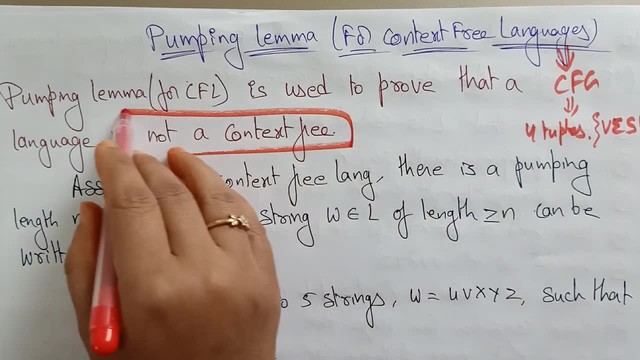 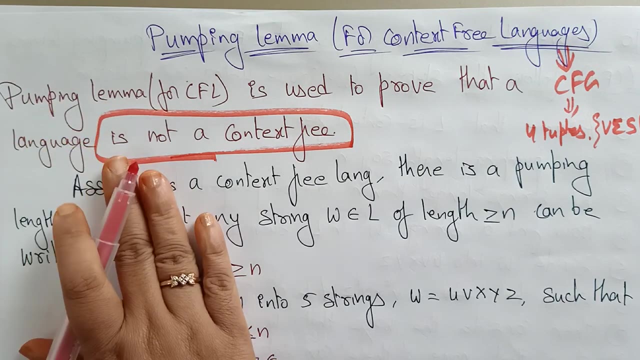 Now, coming to this pumping lemma for context-free language. A pumping lemma for context-free language is used to prove that a language is not a context-free. So the thing here is a pumping lemma. what is the use of the pumping lemma? The pumping lemma is used to prove that the language. 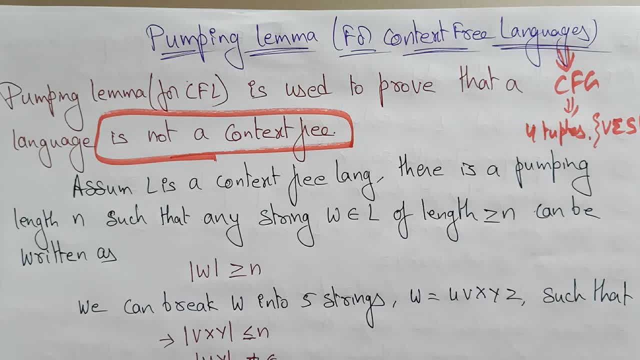 is not a context-free. It is not a context-free Whatever the language that they are given. we have to prove that it is not a context-free. So for this we have to take a first, a contradiction. we have to take means. we have to assume, let us, the given grammar, given language is a context-free. 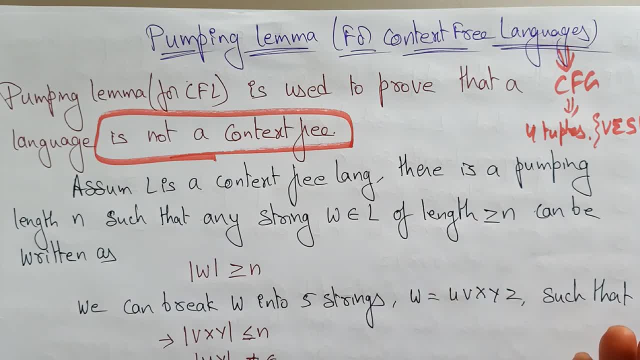 language and try to prove it is not a context-free. So if it is not a context-free means it is a pumping lemma, okay. So that is a way you have to solve. First you need to take the contradiction- We have to assume that the given language is a context-free language- and try to solve that it. 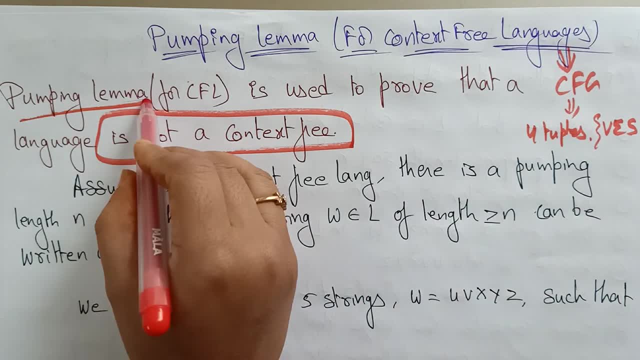 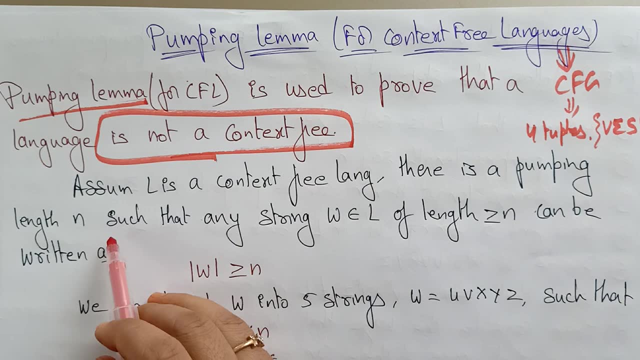 is not a context-free language. If it is not a context-free, then it is pumping lemma, Because the pumping lemma is used to prove that the language is not a context-free language, So not a context free. let let's see the theorem. what is the conditions of this pumping lemma? 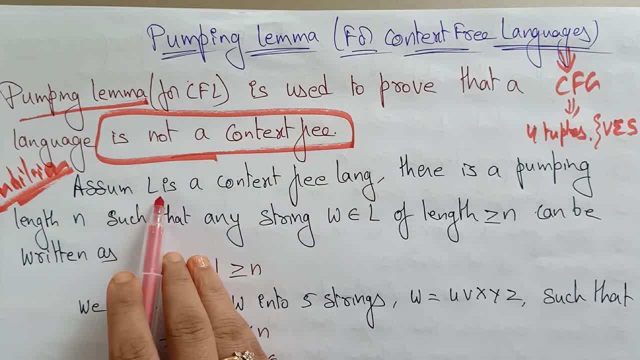 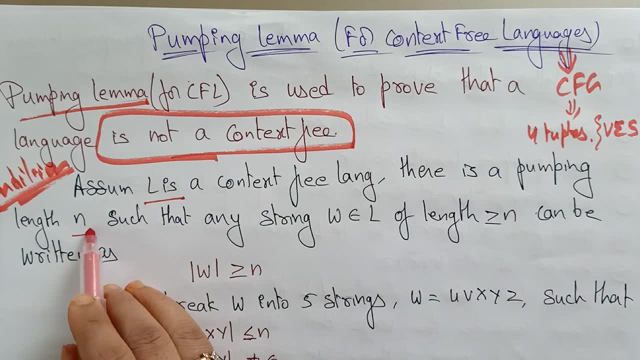 we're showing that is not a context free. assume l: l is a context free language. okay, let us take a language- l, which is a context free language. there is a pumping length. some length should be there. by entering the pumping length, we can identify whether the language is context free. 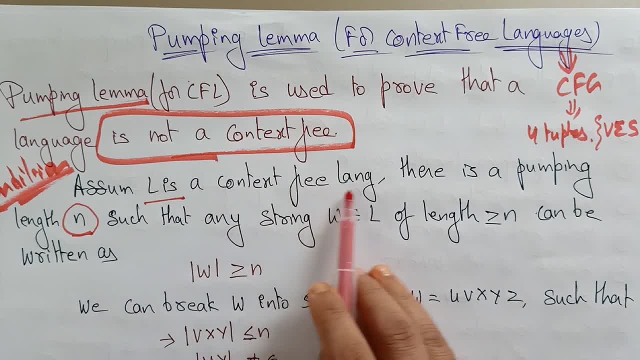 or not. okay, so first assume l is a context free language. there is a pumping length n such that any string, whatever the string that you are taken, okay that any string in the that that string should belongs to the language. okay, that any string that belongs to the language of length greater than or. 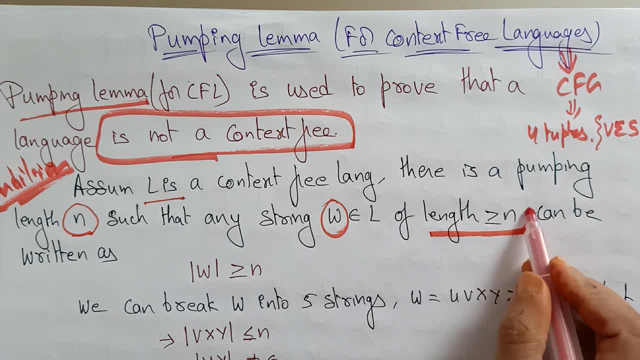 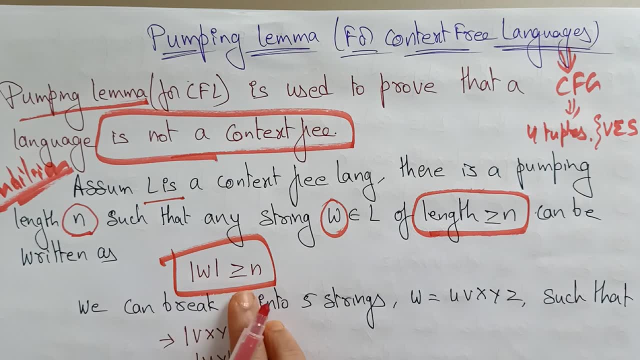 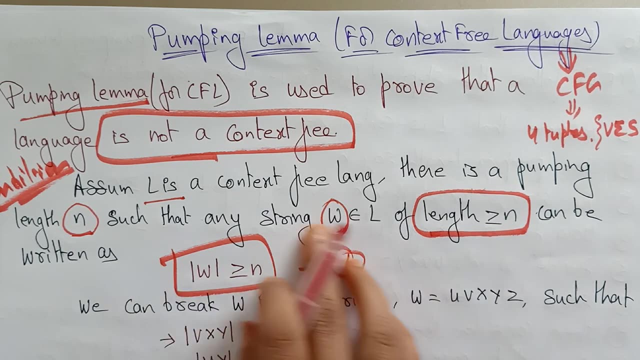 equal to one at the length of that pumping lemma, should be greater than or equal to one n, and can be written as this: more w is greater than or equal to n. there's a first condition and we can break w into five strings. actually this is a condition for that: that the model w, that is, the length of this string, is. 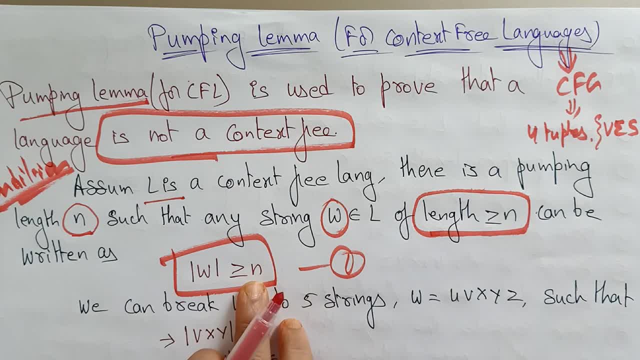 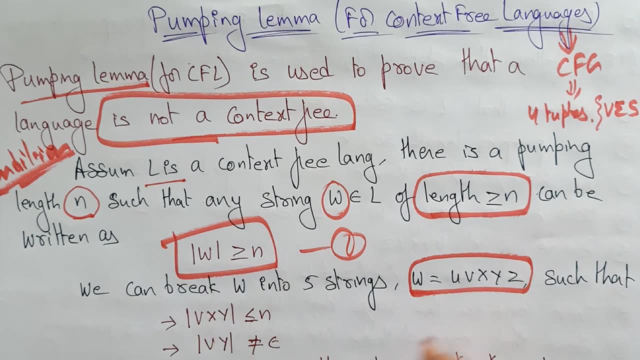 greater than or equal to the given pumping length, n. we can break w into five strings. w is equal to u v x y z, u v x y z, such that mod v x y means this: mod v x y is less than or equal to n and mod. 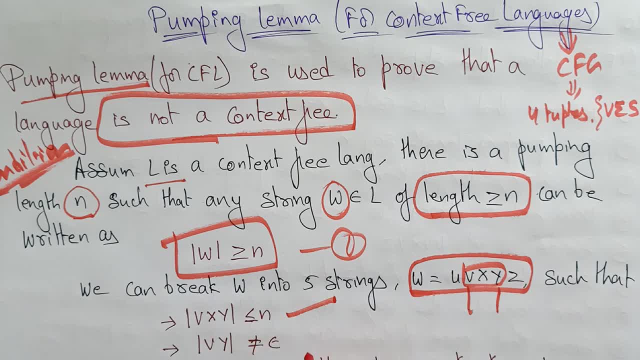 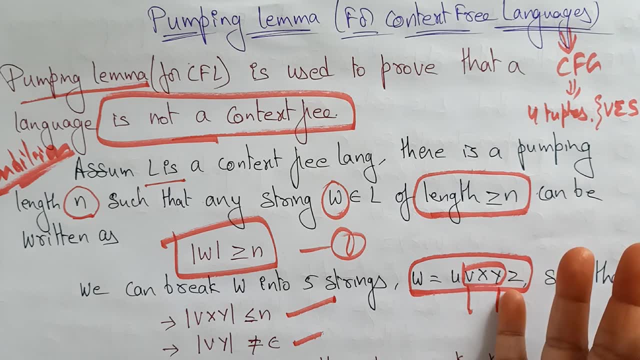 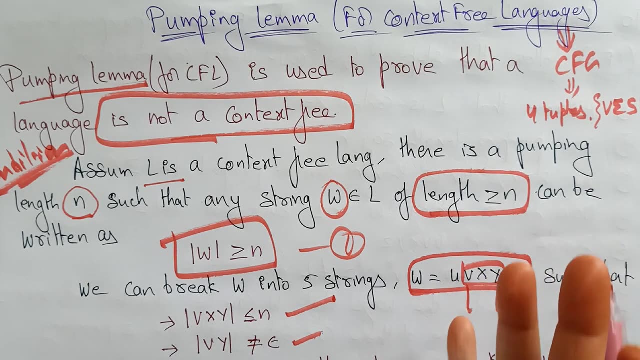 v y. this mod v y is does not belongs to the uh epsilon symbol. it does not be empty uh. it does not be zero because it has. it has a power based on that v y only we are going to decide whether the given context free language is, uh. what a given language is a context free language or not. 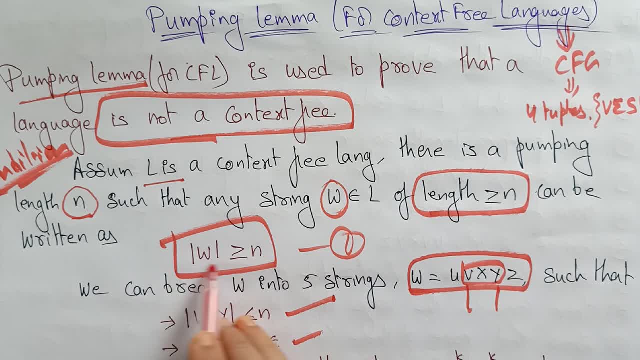 we have to decide. okay, so we break the this string into five strings: u, v, xy, xyz. where v, x, y is less than or equal to n. so these three should be less than or equal to the given string length and mod v, y. this v and y does not belongs to the empty string and for all k. 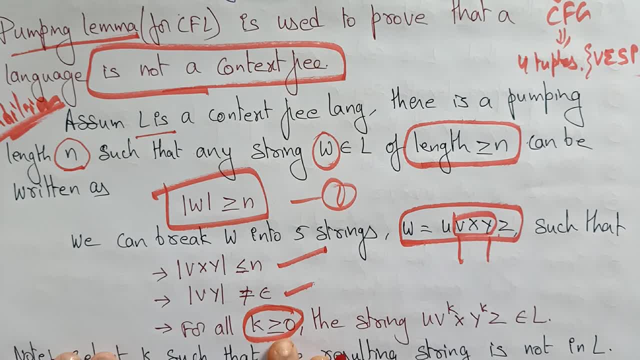 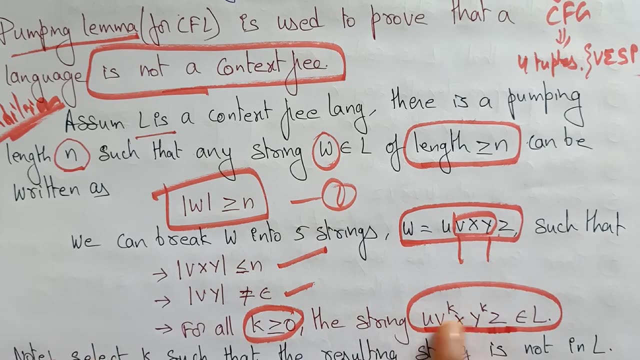 greater than or equal to 0. we have to take a power that should be greater than or equal to 0. the string u, v, power k x, y, power k z belongs to language. okay, if it belongs to the language. so this is a contradiction we are taking. okay, select k. we have to select the k in a way that in the 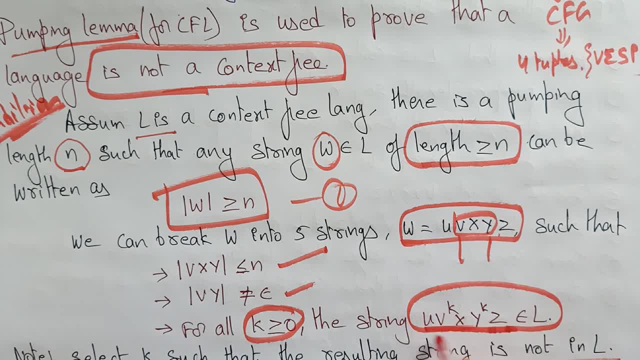 result: the string is not in language. actually this is a condition: v? u, v power k x, y power k z belongs to l, whatever the k value that you are taking, that is, from greater than or equal to 0, if that k value you have to take in a manner such that the resulting string is does not belongs to language. 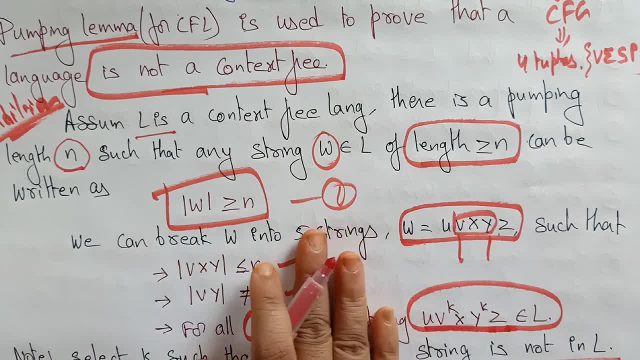 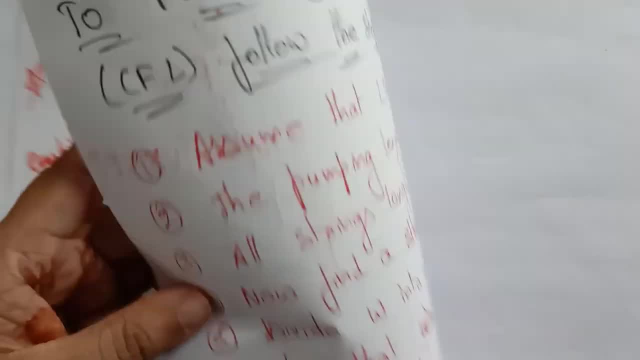 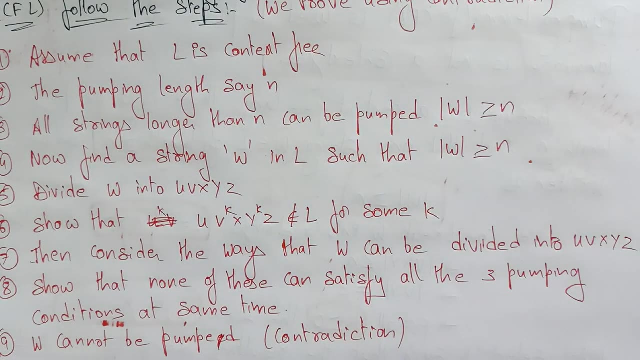 in that way you need to be take. then we can say that the pumping lemma uh is proved, that that the given uh language is not a context-free language. now let's see what are the steps that we have to take. so if you understand the steps, in the next video i'll take an example to prove that the uh. 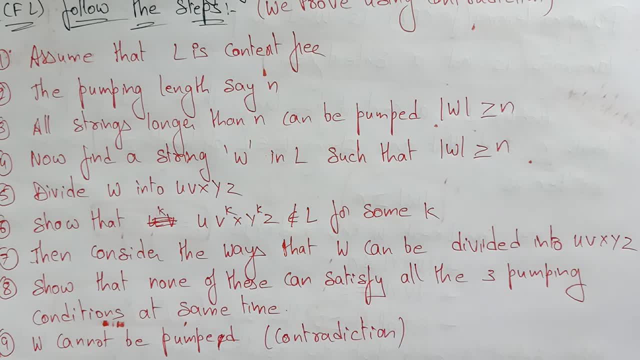 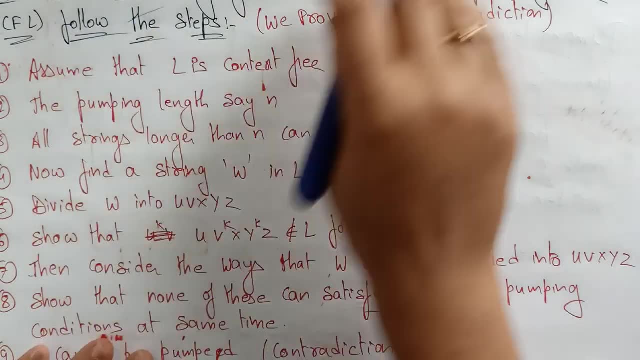 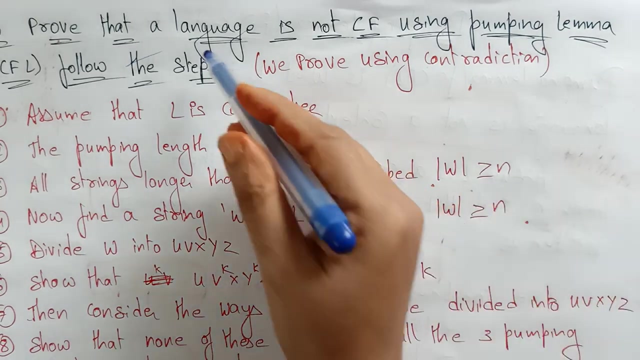 pumping lemma is not a con. it's not a context-free language, whatever the language that is, given that it is not a context-free language. now let's see to prove that a language is not a context-free- context-free using a pumping lemma, context-free language. we have to follow these steps. 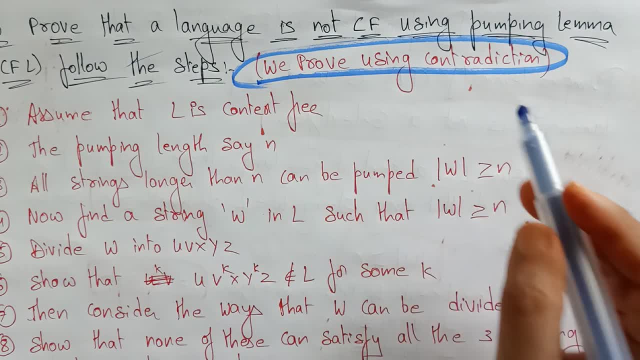 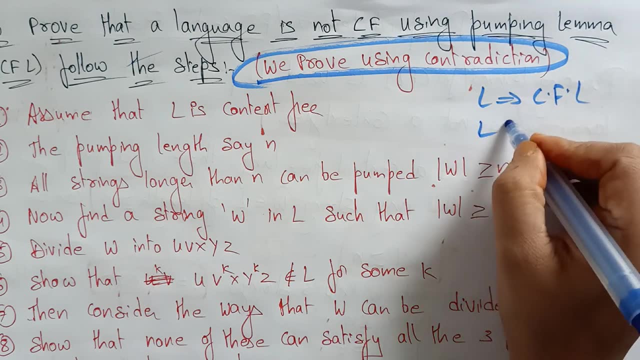 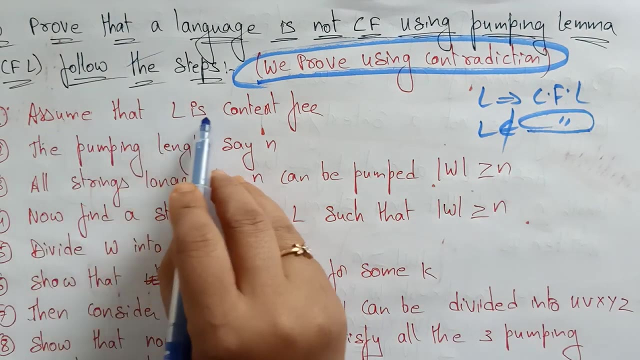 so what i said, just take a contradiction method means let us assume that language, whatever we are taking, is a context-free language and we have to prove that that language does not belong to the context-free language. so first assume that it belongs. to assume that l is a context-free. 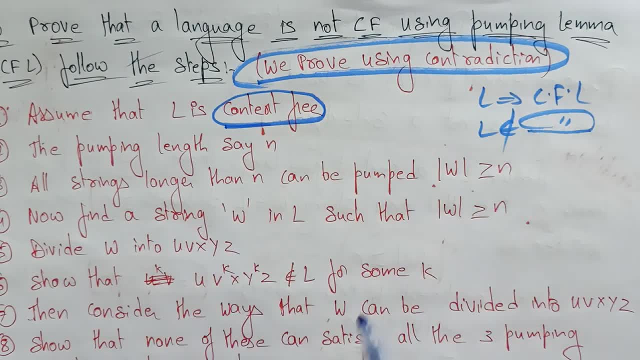 so starts with the contradiction and uh, we, we have to prove using contradiction method. so i had started with the contradiction. i am assuming that the given language is a context-free and i have to prove that it is not a context-free. there is a problem? uh, solution. so the pumping length: 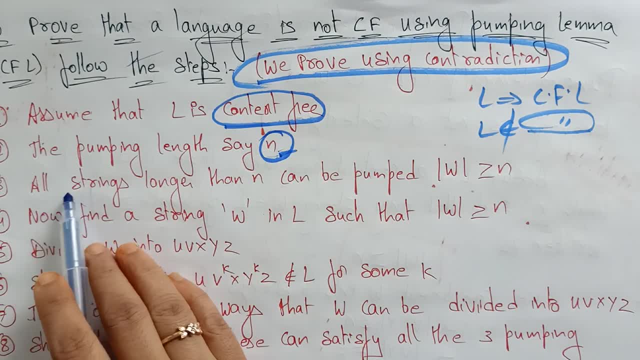 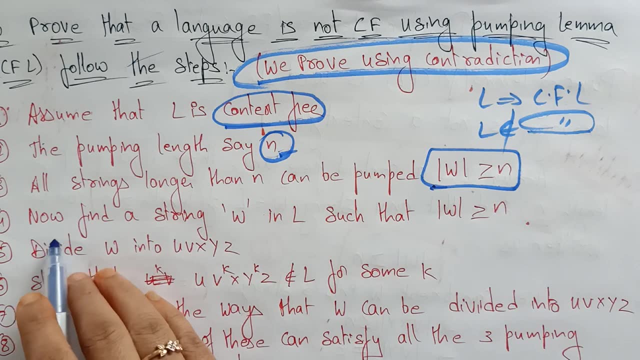 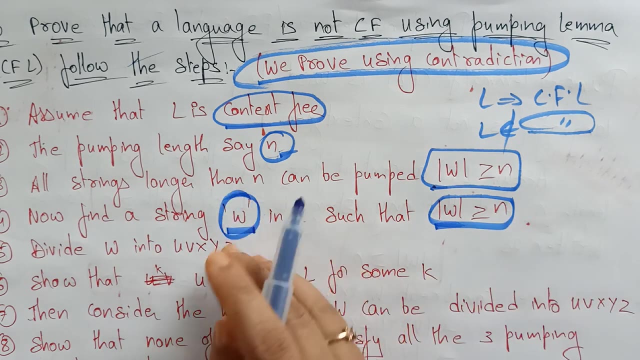 say n. let me take some pumping. length is n and all strings longer than n can be pumped into more. w is greater than or equal to n, according to our condition. Now find a string w in L such that w is greater than or equal to n. So whatever the string that